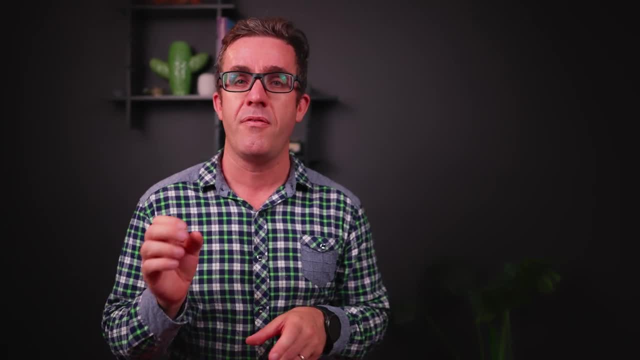 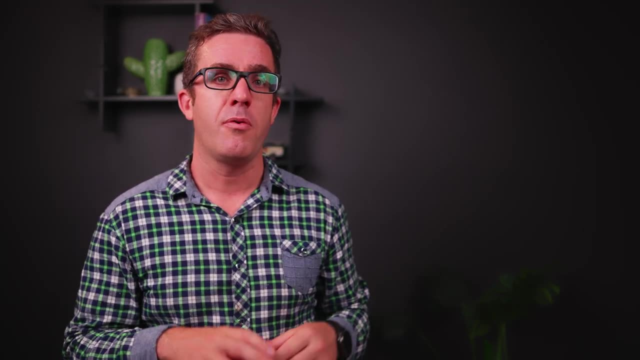 The soil that you're going to be founding on will likely dictate the type of foundation system that you would choose, as the different founding materials will behave differently under different loadings and different conditions. So before you start any project, it's important that you get a 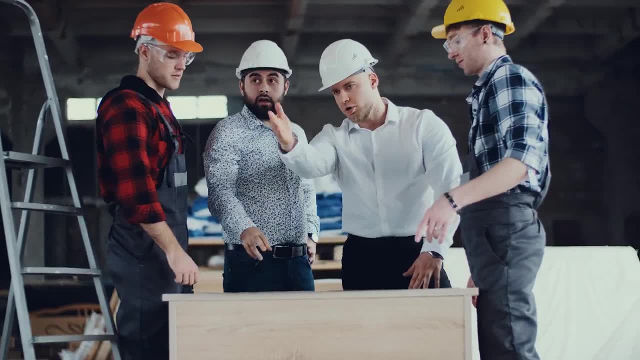 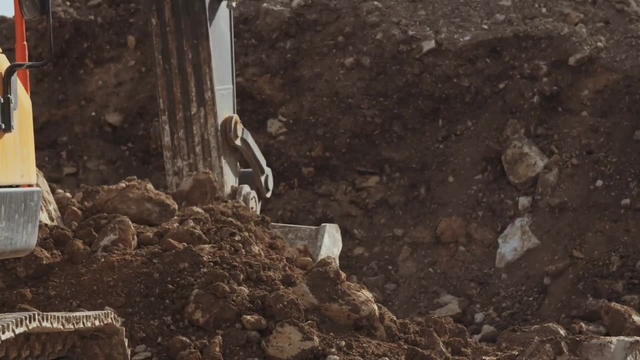 geotechnical engineer out to site to investigate, to look at what the founding material is underneath and how it's likely to behave. The subsoil structure will not only vary between your different locations, but it can also vary across the site if you've got a large. 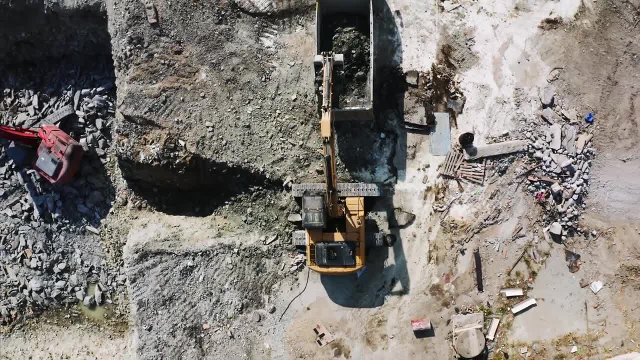 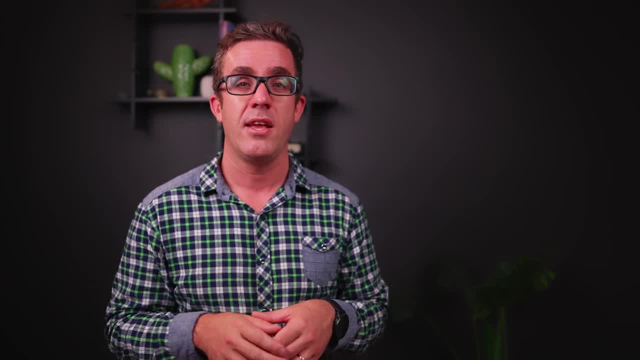 building, so you may have one type of soil on one side and a varying material on the other, so it's important that you test the whole site. The subsoil structure is likely to be a combination of the primary soil types, and these come in a number of different forms, So either have your clays, which 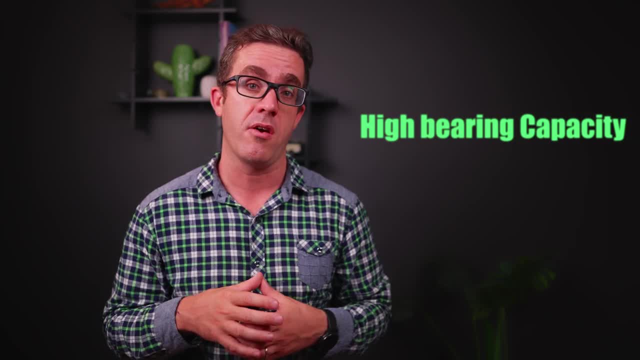 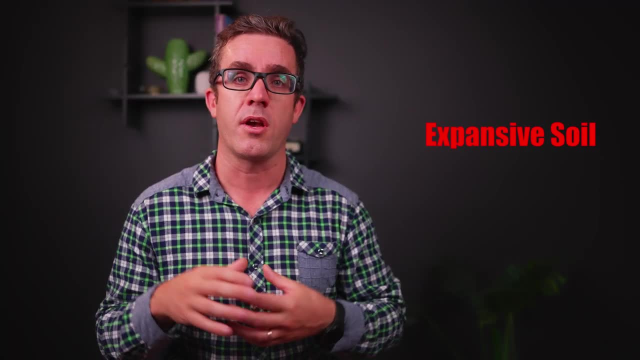 is a sticky, expansive material which you can get some quite high bearing capacities out of. but once it gets wet it will swell up and move. so your foundations need to consider the expansion and contraction of a clayey material. Have your silt, which is still a little bit sticky. it's a little bit softer, though it does expand. and 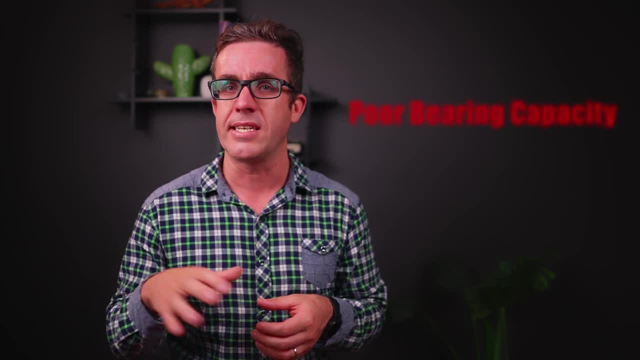 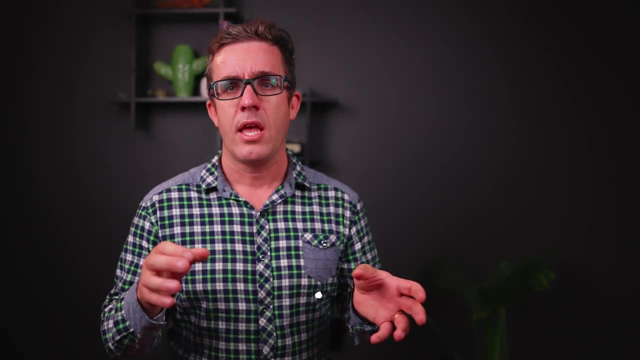 contract but has generally really poor bearing capacity. then you can move into your gravels and sand, which is more of a coarse material. they don't really behave that poorly when they get wet. they may have a poor bearing capacity. as you press down the soil particles may move away. 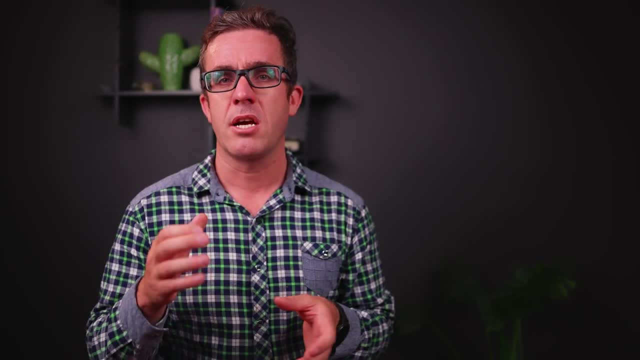 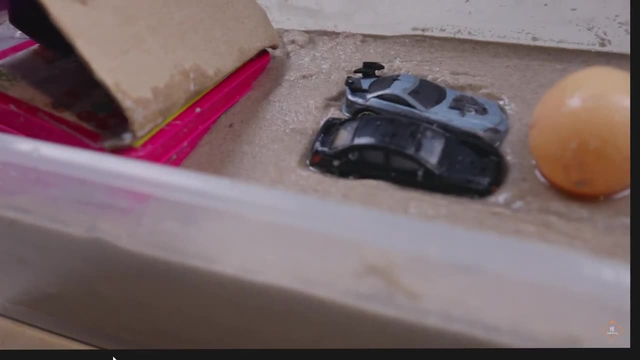 The other problem of a coarse or sandy material: they can be subject to a liquid faction event. now I've done this in previous videos. but when it gets wet and you shake that material, the soil can turn into more of a liquid, sinking the building into the ground and, of course, the best material. 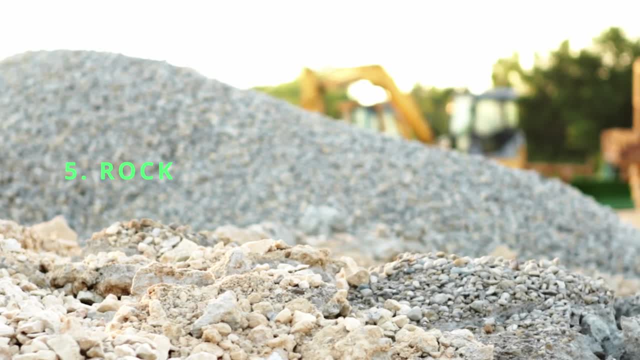 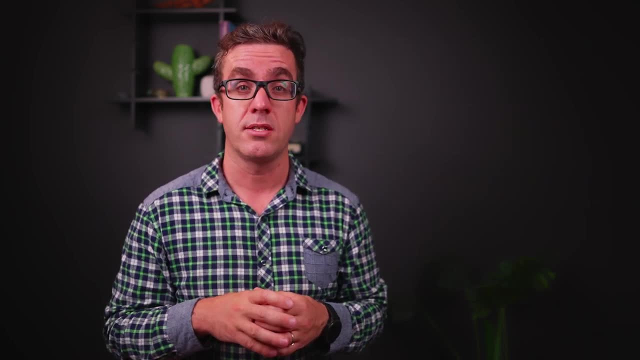 that you can possibly get is that rock. now, rock is really solid so it has generally a high bearing capacity. so generally, if you're finding on a rock system, you'll likely have the most cheapest footings. but you do need to be careful about the rock as it could be either very fracturous. so when you put it on, there could be a lot of movement. you can also get a variety of strengths. you can have your soft sandstones all the way up to your hard basalts. wherever possible you want to be trying to have the highest bearing capacity. then typically sand is your next cheapest, as it doesn't have that. 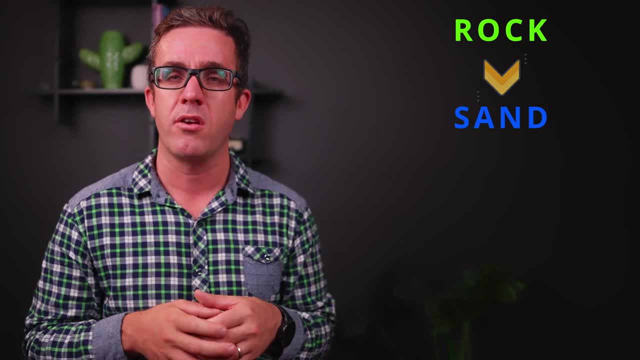 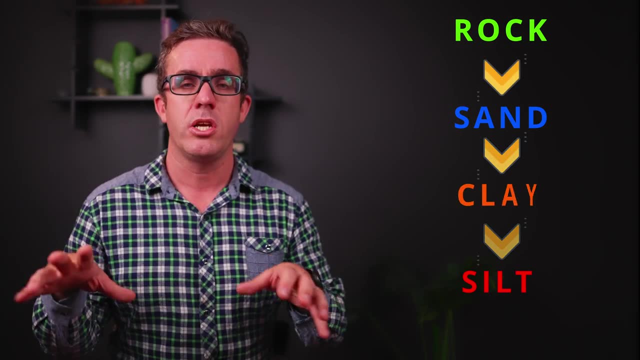 contraction and expansion, you can still achieve a relatively high bearing capacity. silts are generally your worst as they have that soft material, so typically you'll need some sort of piling system. then clays just need a really stiff footing system, as you can get a high bearing. 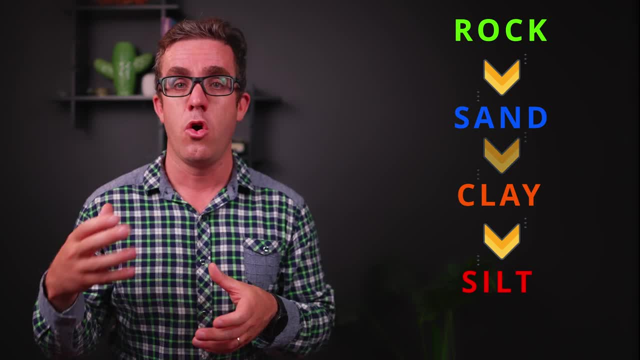 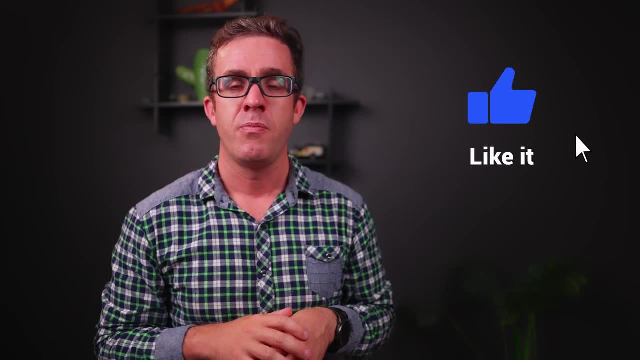 capacity, but it can well and contract under even just normal moisture differentials from seasonal movements, much like the footings bearing down on the soil. don't forget to bear down on that like button. not only does it help my channel out, but also let me know in the comments below if you. 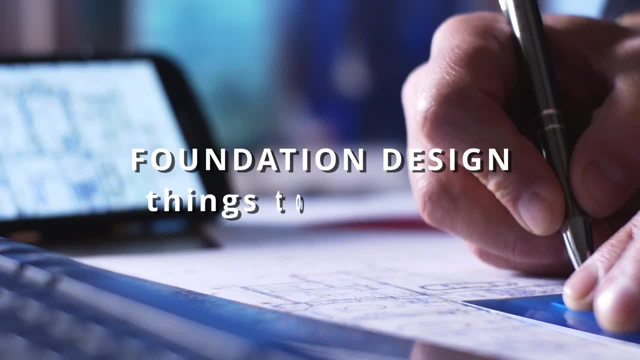 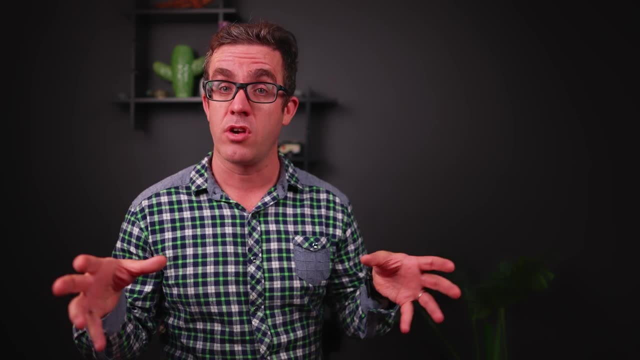 have these channels to get out to more people. so what's other things that you need to consider when you're looking at your foundation design? we just talked about earlier about how stiff your footing system needs to be. so if you've got a highly expansive and contractive soil, the footing system- 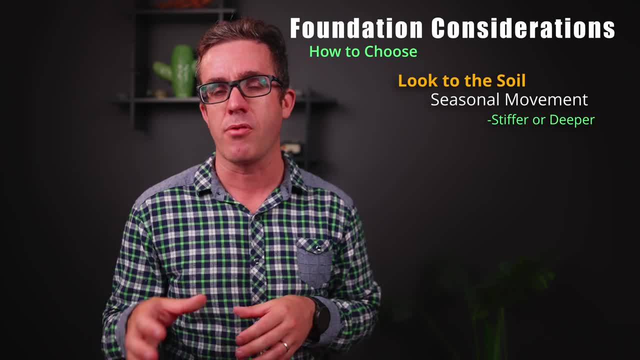 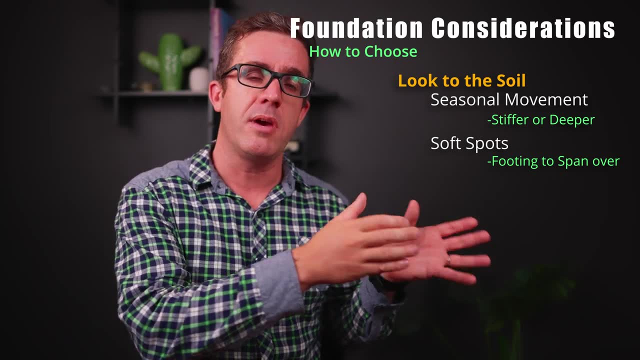 needs to account for that movement and be stiff enough that it doesn't break under those seasonal movements. you can also have different soft spots across your soil system, so if you've got certain spots in areas, you may need to span across them. so the footing system may need to span across the. 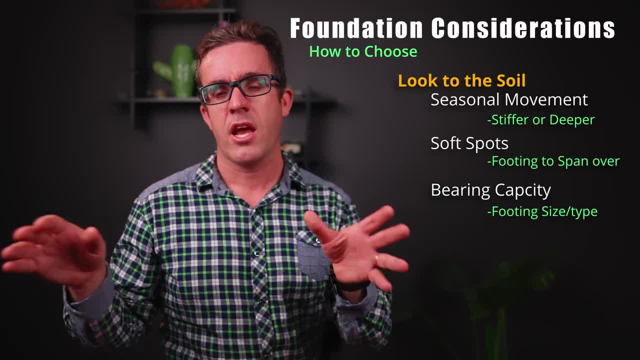 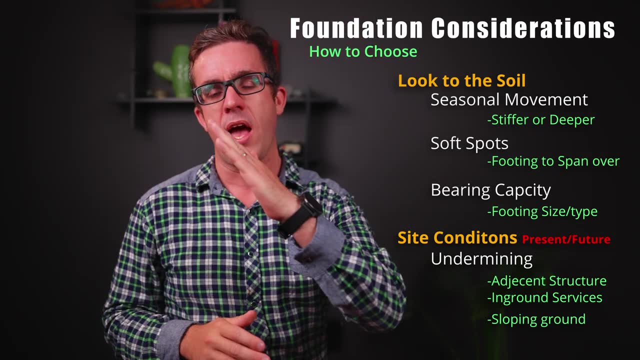 soft spots to get to the solid material on either side. another careful consideration when looking at your footings. sometimes you may have a varying height, as you may either have a basement or sloping block, and soils do have an angular repose, so the angle at which they 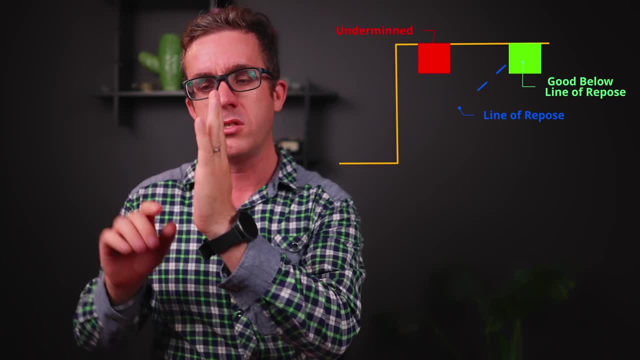 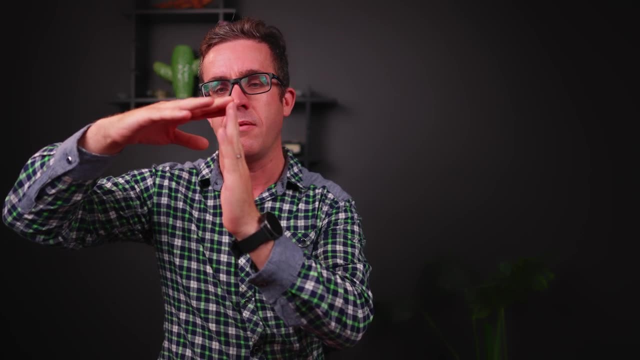 generally want to slope at. and if you go beyond that angular repose you're typically undermining the footing system. so this footing up here can't bear on the soil underneath. it has essentially lost its bearing capacity. so if you are undermining it, the footing system needs a coat for that area. 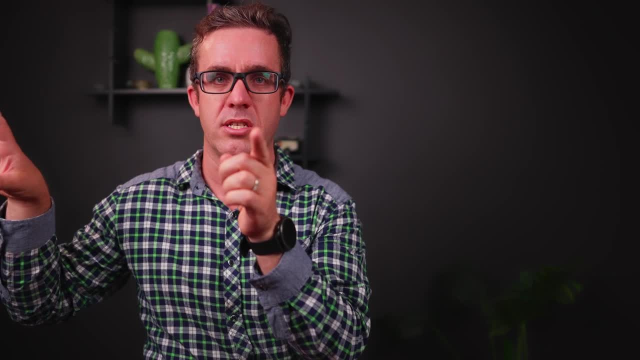 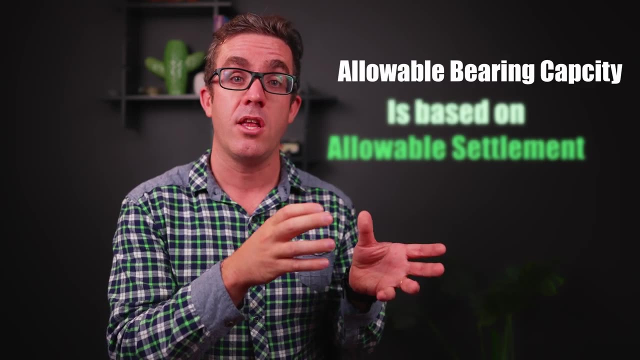 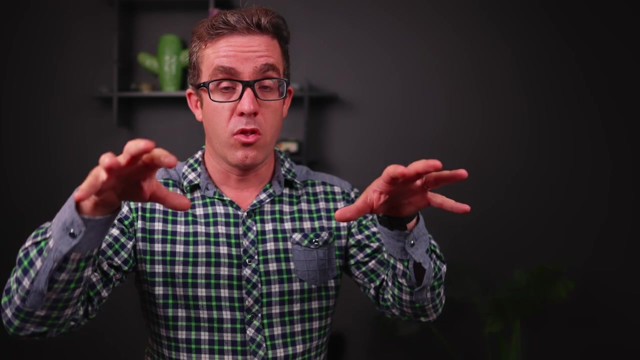 which you've undermined so we can go to the more solid foundation system further away. any foundation design is governed by the allowable bearing capacity, and this allowable bearing capacity is calculated based on the allowable settlement of the structure. as we know from newton's first law, any action has an equal and opposite reaction when load goes onto. 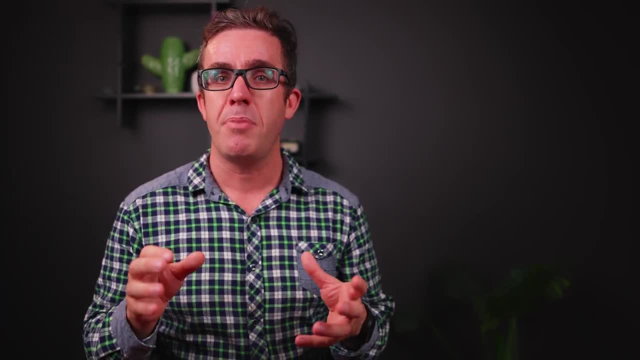 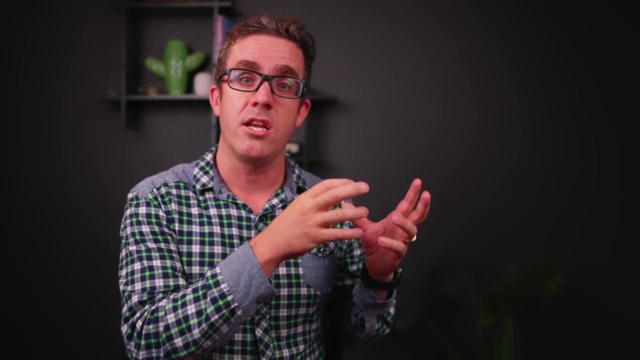 the ground it will settle to some extent and the bearing capacity is based on this allowable settlement. so depending on how big a smaller load you can have, that allowable bearing capacity that you get is based on the allowable settlement of the structure. now i've gone through some of the 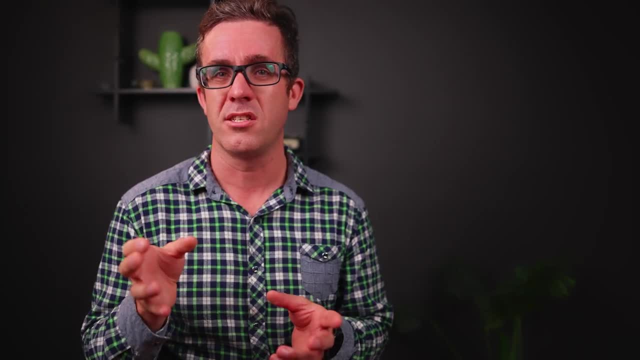 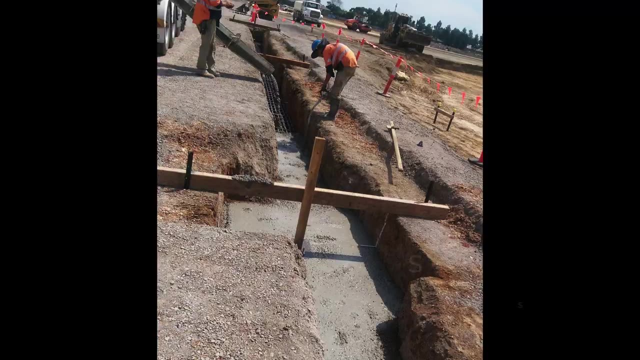 things that you need to consider before even getting into the selection of your footing systems. what type of foundation systems do you have available for your footing system? have available to you so you can either have a shallow foundation system, which is more like your pad footings, strip footings or rafts, or you can have a deep foundation system, which is either 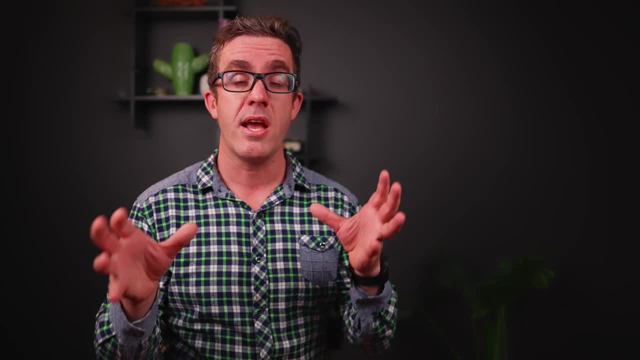 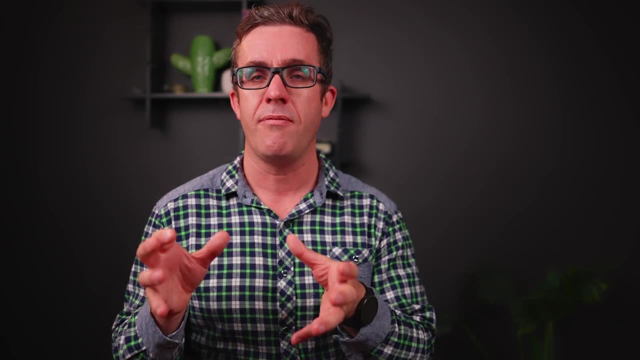 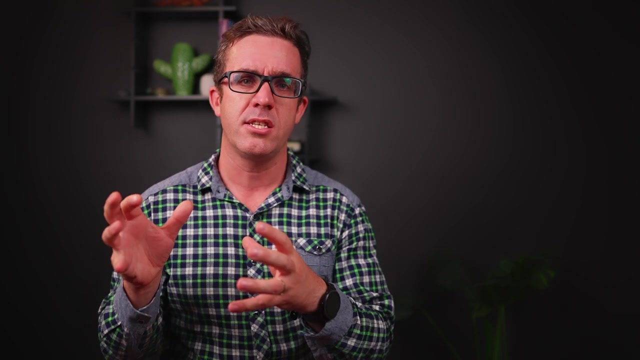 your driven pile, screw piles or pile foundations. now you may have a combination of these in your project, but typically you don't want to mix different founding materials, so you don't have shallow foundations mixed with deep foundations, as the deep foundations will move less, potentially causing a differential settlement problem. so if you're founding on one type of foundation system, 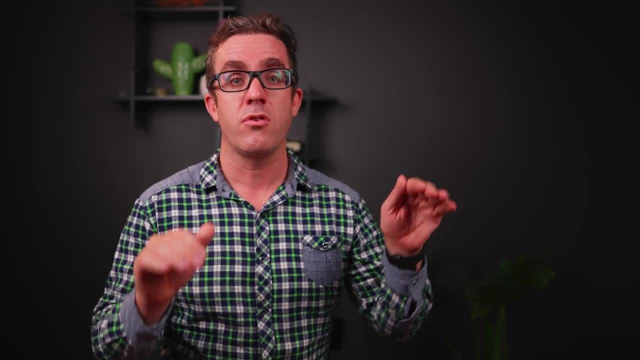 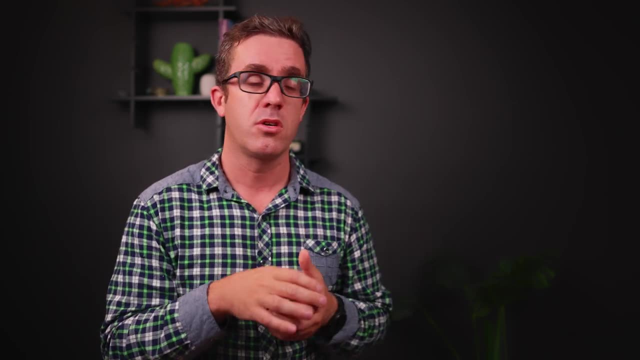 you want to make sure that you're picking one or the other, or having it such that that differential movement will not cause issues to your structure. so what are the benefits and drawbacks of using either a shallow or deep foundation system? because surely the deep foundation system is better? well, no, because you're going to spend more money, potentially. 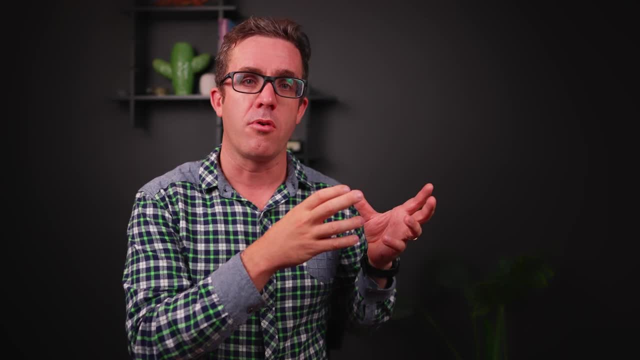 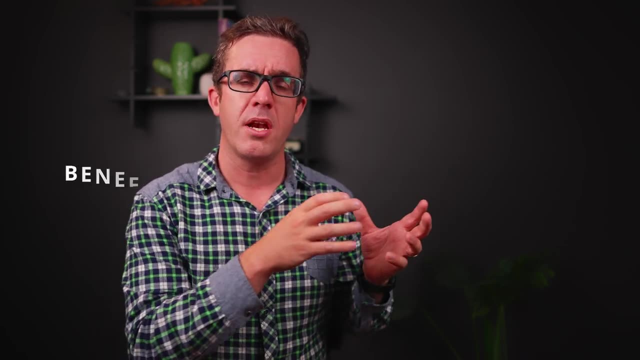 when you don't need to, where the shallow foundation system is normally your cheaper option. so, wherever possible, you want to try and pick that shallow foundation system if your structure can cope with it. so what are the benefits of using a shallow foundation system? as we're saying, it's typically cheaper, it's easy to build as you just need to dig down and bear on. 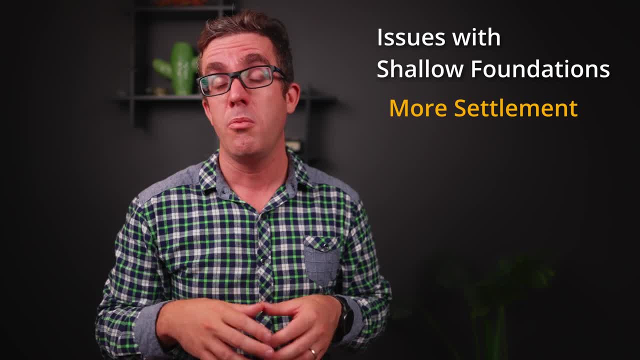 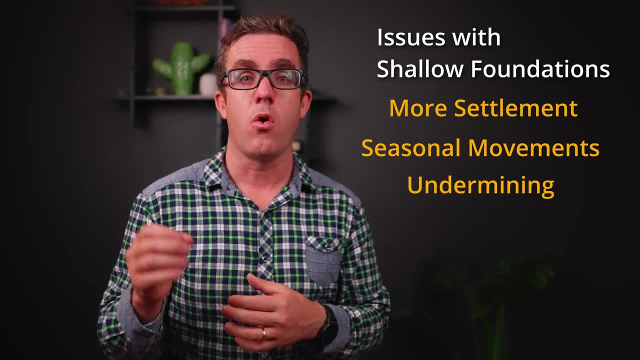 soil below it. the other problems is: potentially you will get a lot more settlement. it will be more subject to those seasonal movements. it can potentially be undermined by either adjacent structures that need to get built earlier or after, or if you've got deeper areas. so if you've got one. 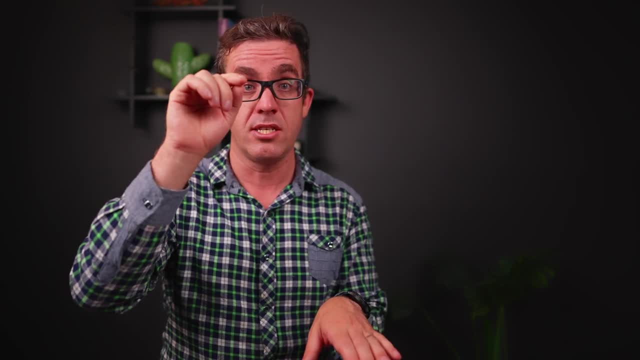 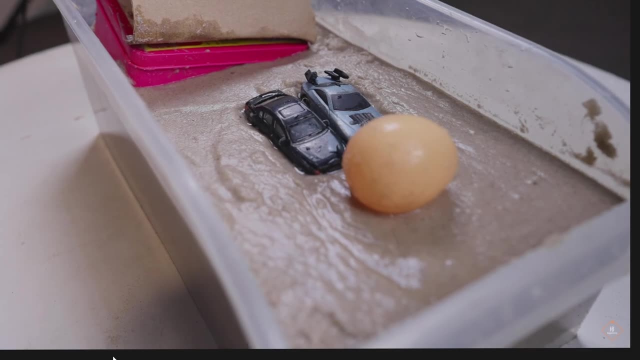 area that's founded on one location and you have a shallow foundation system close to it, this may cause a problem. the other issue, as we're saying before, was that liquefaction. so your shallow foundation systems are typically subject to that liquefaction problem. so if you're in the wrong area, 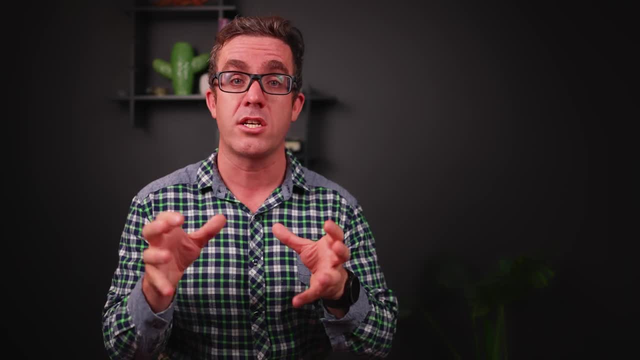 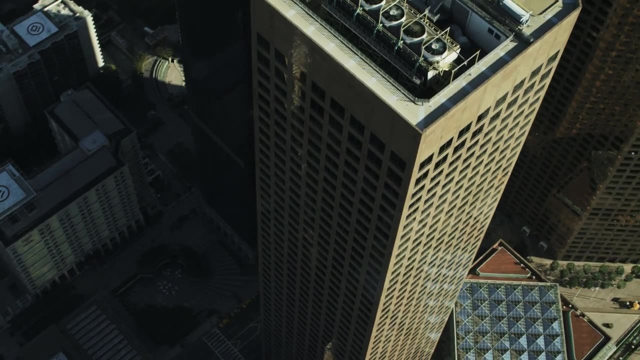 and you want to build a shallow foundation system. you might want to build a shallow foundation system that's not going to have enough bearing capacity but for its capacity underneath an earthquake and that liquefaction event. where you want to use your deep foundation systems is if you've got loads that are way too high, for example, if you've got a high load from a building. 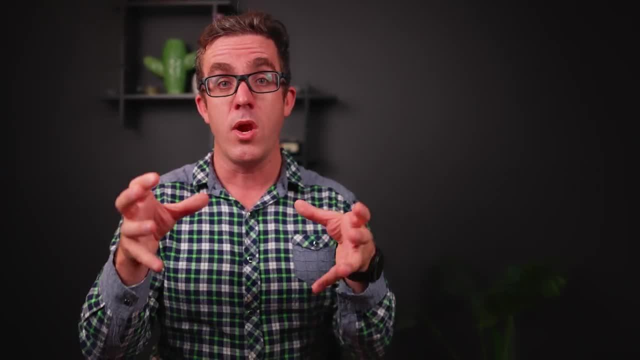 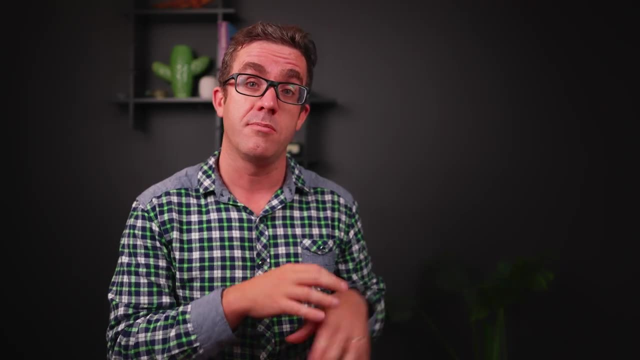 coming over and there's not enough bearing capacity in the subsoil structure that you'd be founding on, you might put piles down to the bedrock below if you've got uplift problems. so if you've got a really high wind uplift and need a lot more mass in it, a pile can be quite a good option to. 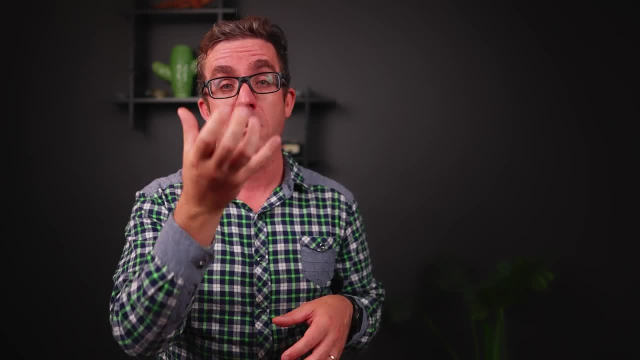 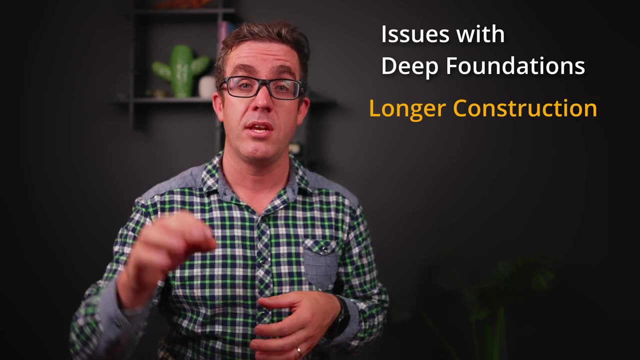 tie down that building or if you've got really poor foundation systems such as that silt. so if you're some sort of piling foundation to get below the silt and onto the better bearing capacity below, now the drawbacks of the piling foundation system: it is longer to build as you need to install the. 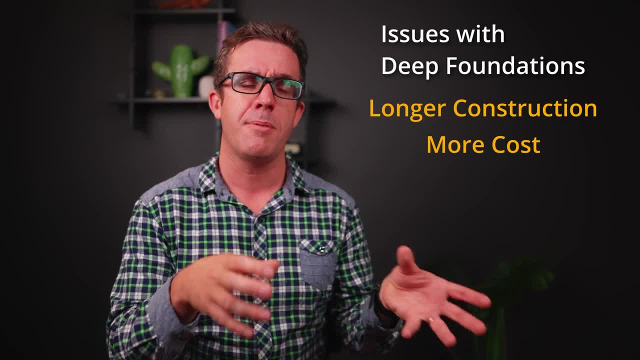 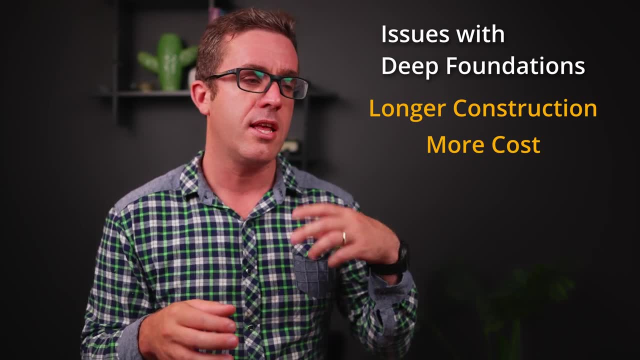 piles. there's a certain trade that you need to bring in and typically, when you're installing your piles, you're still installing them with some sort of pad footing or strip footing to spread the footings around. so you not only do you need that same foundation system you've got on your shallow. 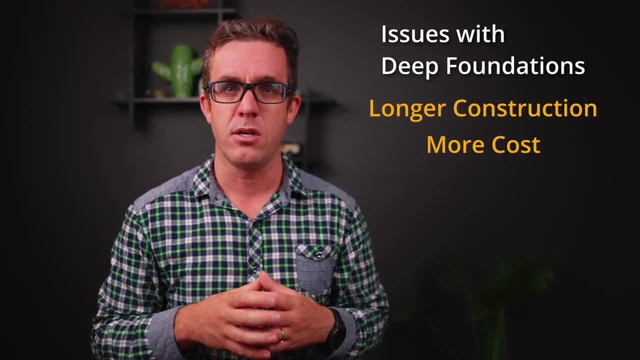 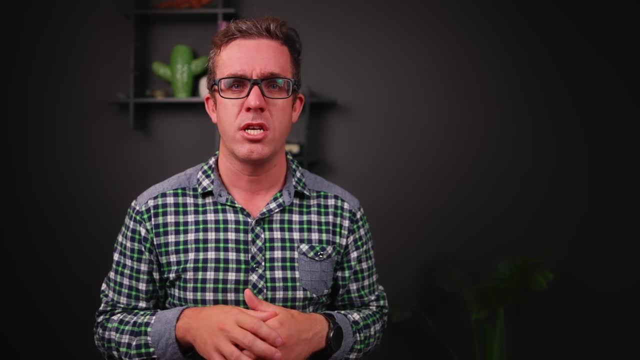 foundation system, but you also got the pile structure integrated in your design as well. but really, where it shines is, it's not subject to much of that seasonal movement. you can drill the piles down deep enough, so it's not subject to that moisture change. again, if you've got that really poor foundation system, you may need to choose it, or you know. 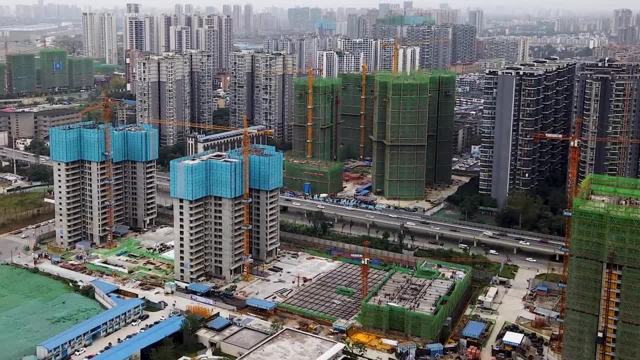 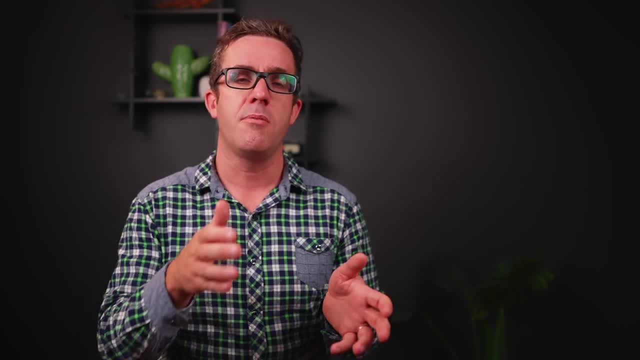 there's going to be a future development next to you. potentially, when they dig down and move the soil away, they'll either draw down the water table so that deep foundation system won't be affected from that future development or potentially undermining it if you've got a shallow foundation. 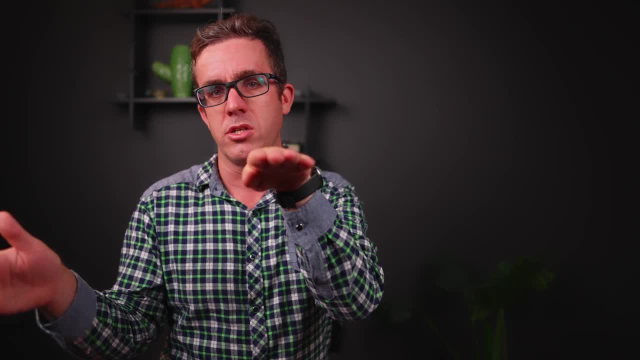 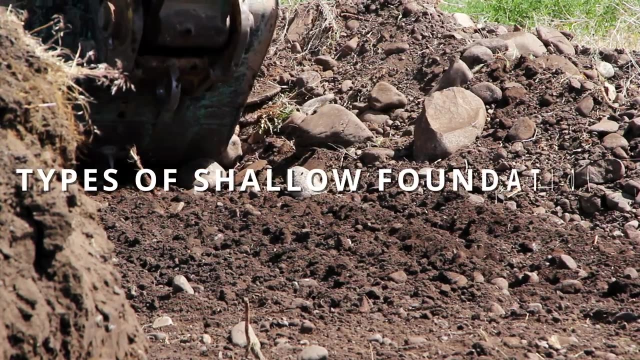 system. you've got the building next to you. you dig down. they haven't undermined your footings. so just some things you need to consider when choosing either a deep or shallow foundation system. so what are the types of shallow foundations that you have available to you? so you either have that pad 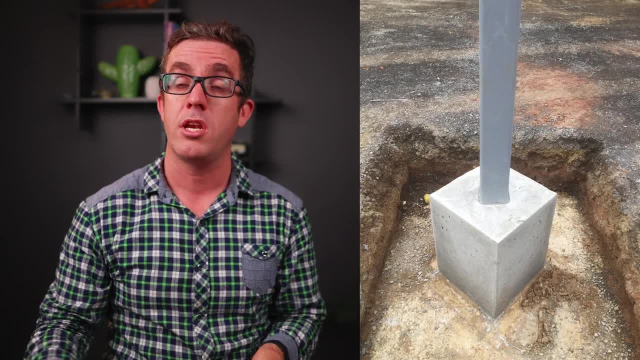 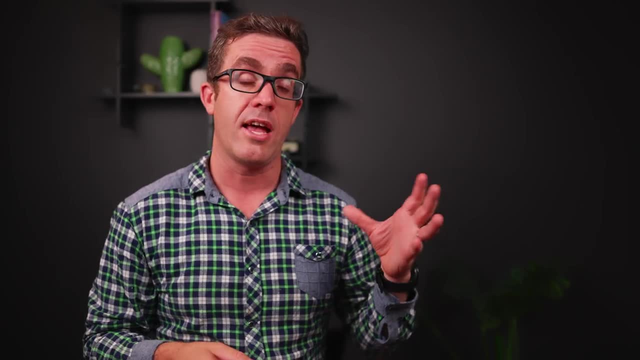 footing, which is your most common type. now. pad footing is just an isolated pad, typically with a point load from a column over the top. that pad footing is sized based on that nominal load that you need to spread it over, so based on the allowable bearing capacity from the geotechnical 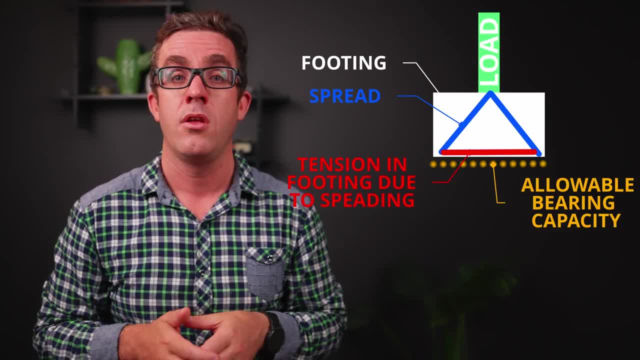 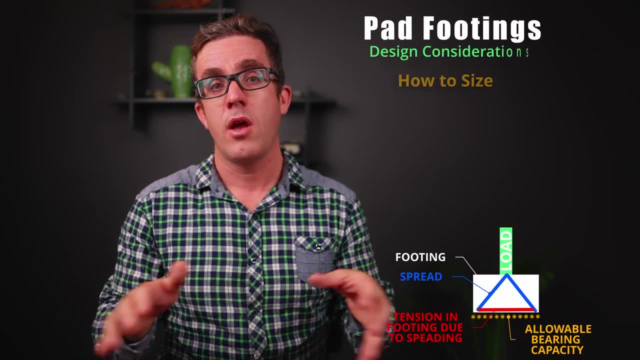 engineer, then you just need to design the load for that strut and tie action to allow that load over to spread across the area underneath it. some things you need to consider when looking at that pad footing: does it spread out at the right angle and what is that tie capacity in the? 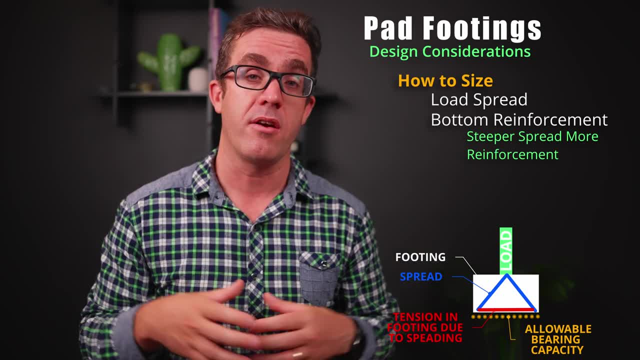 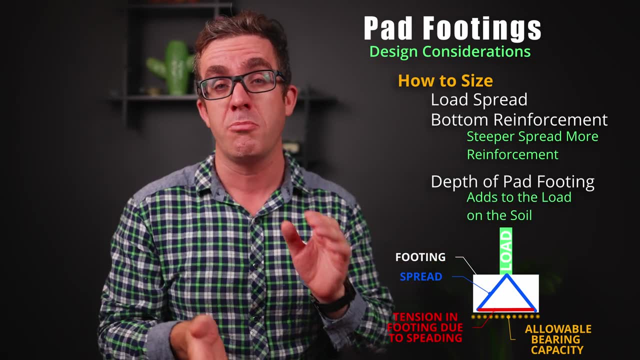 bottom of your pad. have you spread the load far enough to get to that allowable bearing capacity? and what a lot of people often miss as well is the pad footing actually is adding weight to the soil. so if you've got a shallow building, the pad footing would be quite significant to the load that 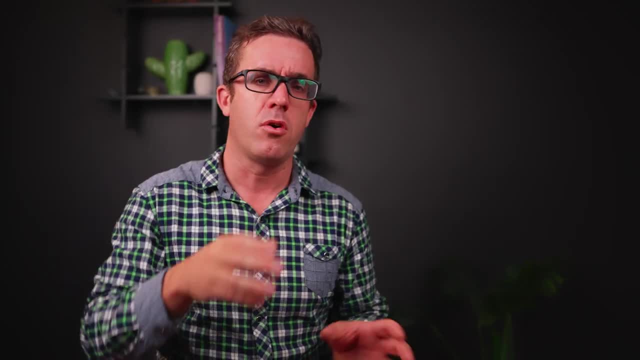 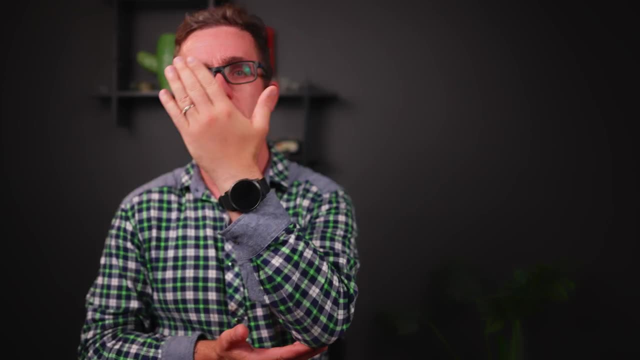 is applying to the soil as well. so not only do you need to consider the load over, but also the self weight of the footing system itself, so you can also have pad footings that may need to be rectangular in form. for example, if you've got a column up and it needs to resist lateral actions, the footings 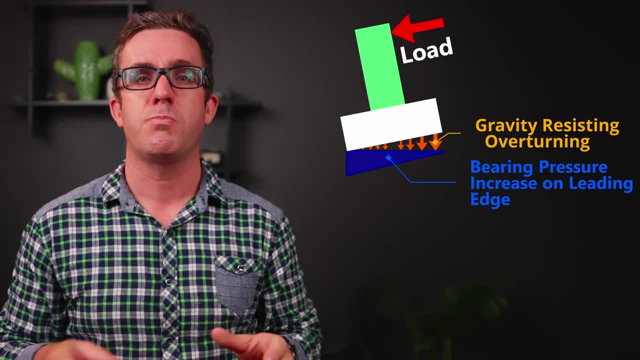 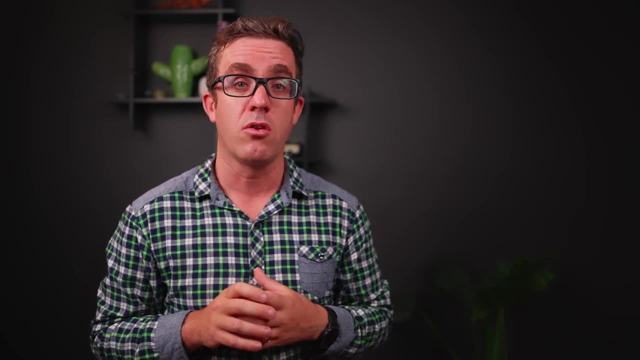 need to have enough weight in it to kind of balance that movement but also spread out the load. the next type of foundation system, and likely the second most common footing system that you're likely to encounter, is a spread footing or a strip footing. a spread footing is typically just. 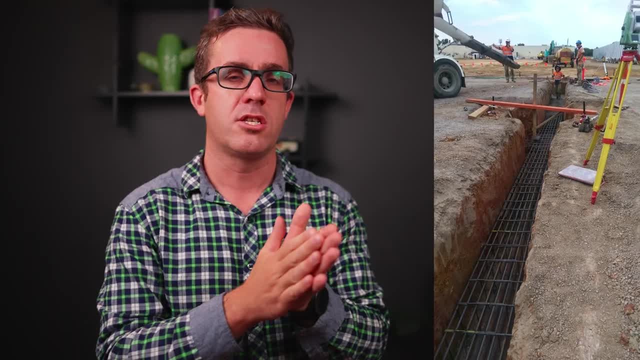 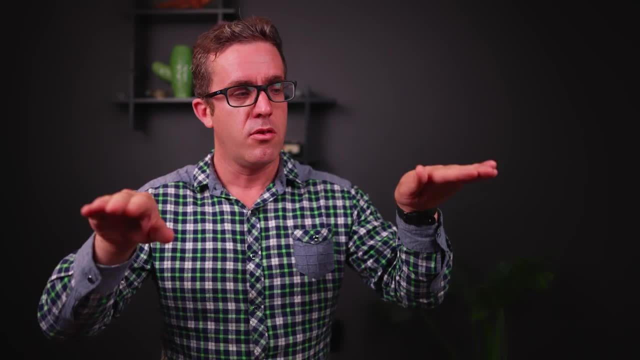 a beam that's cast into the ground along a long length. this can either support line loads from walls over, as it will spread the load across that length. if you've got differential movements and you need to tie things together, you generally have that beam and it'll typically balance out the 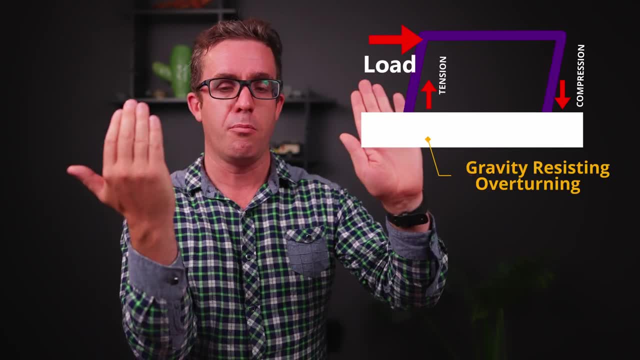 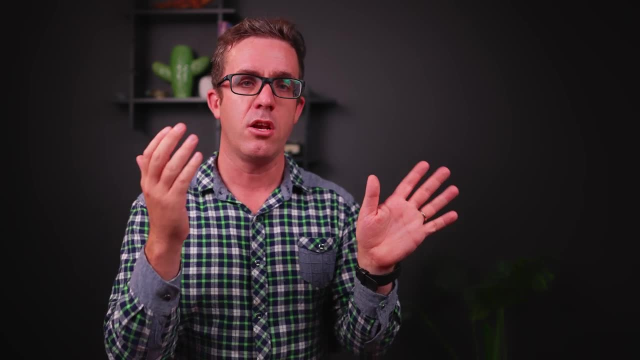 movement in the structure. those strip footings also really good, as if you've got a frame that you need to resist overturning, as you can have the beam connecting to balance out the forces. so a variety of different purposes that you can use your strip footing system for. 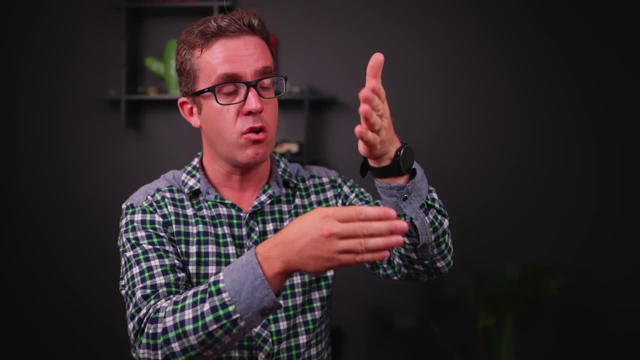 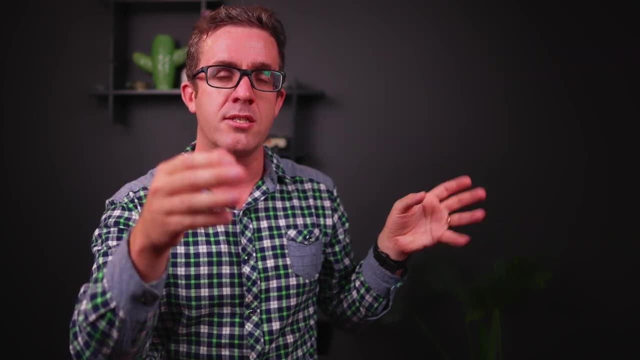 the other benefit having strip footing is if you've got surfaces cast into the ground or soft spots, so typically surfaces can't take a lot of load from the structure over the top, so you need some way of spreading over those locations. it's also good for going over soft spots, so you've got soft. 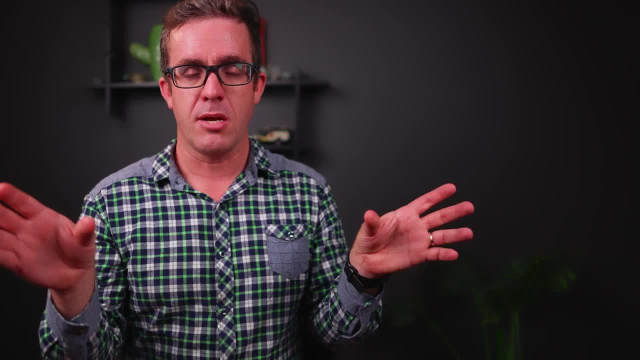 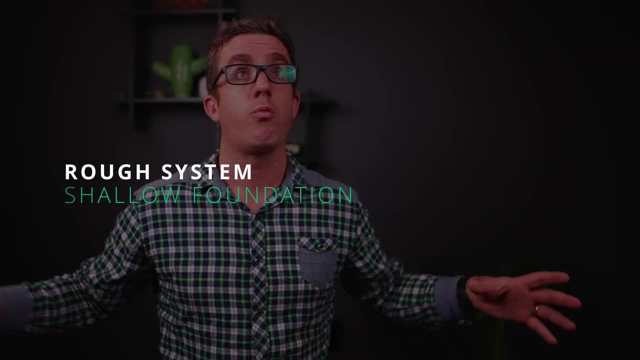 material in between and the footings need to span over it. the foundation can be designed to span over that soft spot and go to where the good material is. the other one is a big raft system. so, for example, if you've got a really big towering structure, 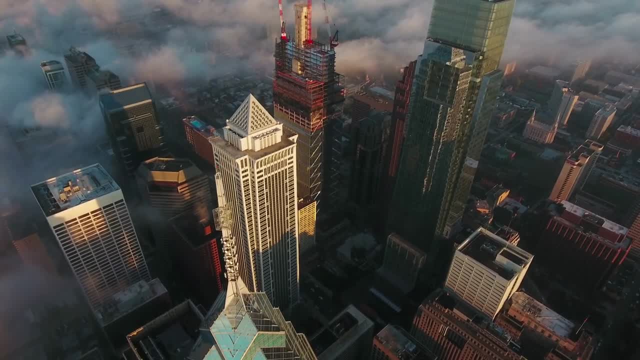 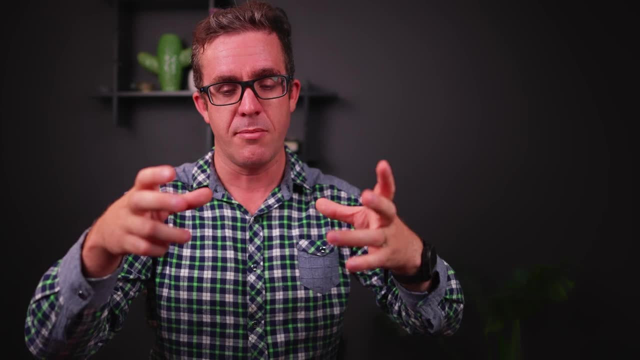 above you and you need to put the loads onto a single footing system, so you typically have multiple walls or multiple columns. the raft is typically a lot bigger, covering a whole core, for example, so you've got a core structure coming down that has big overturning moments and 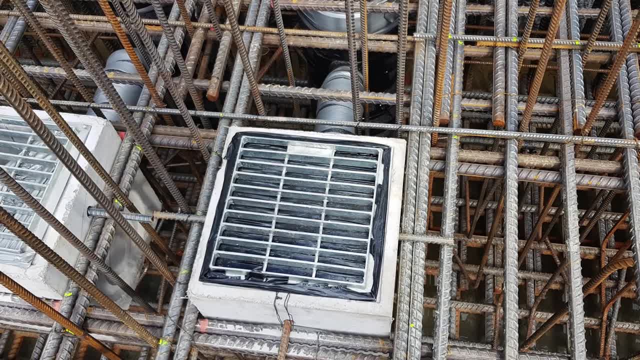 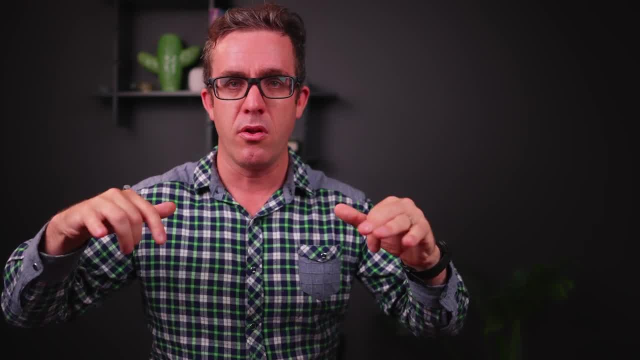 movements that it may need to resist. typically they're quite deep to get enough mass in them to resist those overturning loads. it can also help with differential movements. if you've got a big, big raft system and multiple point loads on them, the system will act as one as opposed to just. 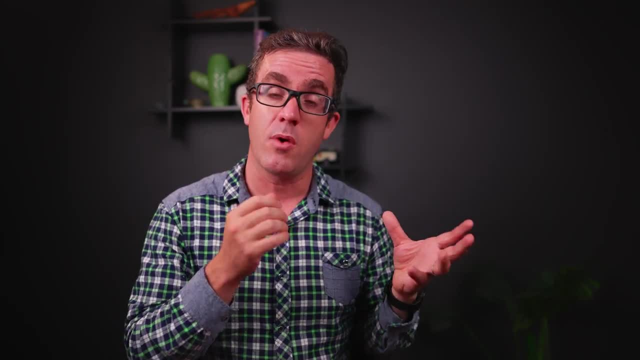 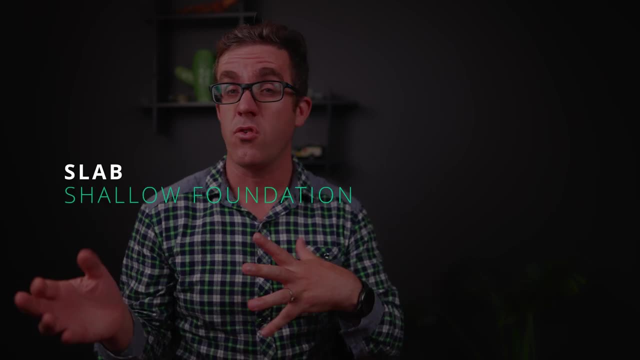 isolated pads, or if you've got soft spots and you don't know, potentially, where they're going to be, so the raft can span in whatever direction it needs to to get to the correct bounding material. you may also have a slab integrated in your design, so you can have things such as waffle pods, which 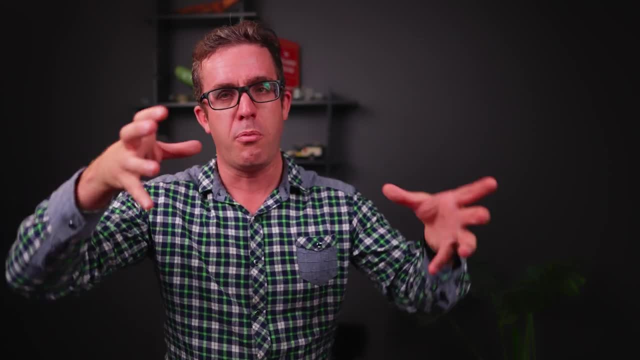 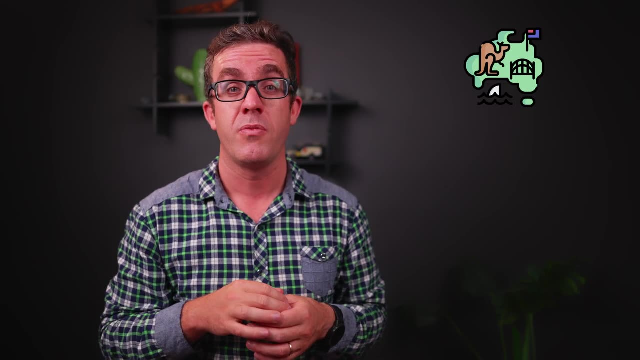 is really stiff, so in that highly reactive soil the waffle pod can move up and down and be quite effective at resisting those actions. or typically the most common one, especially here in australia, is that stiff and rough, so you'll have edge beams around the outside and ridge beams internally to. 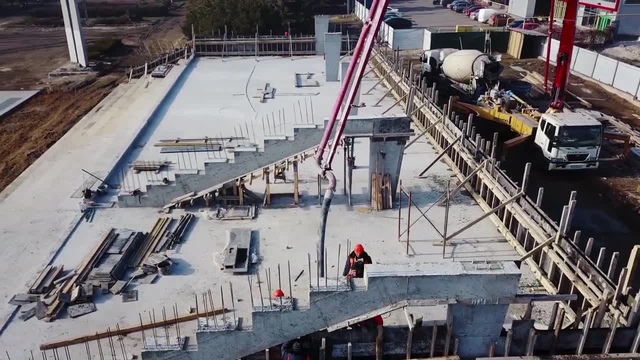 not only stiffen up the slab. so when it does get that differential movement, there's enough stiffness in the slab to stop it. the other way around is, if you're going to have a lot of really good thing about that stiffen raft and with those edge beams, is that you can modify it. 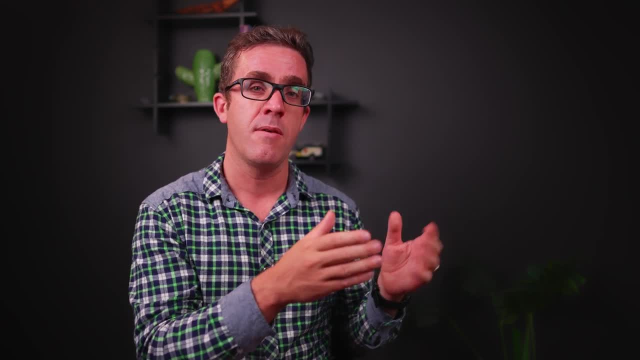 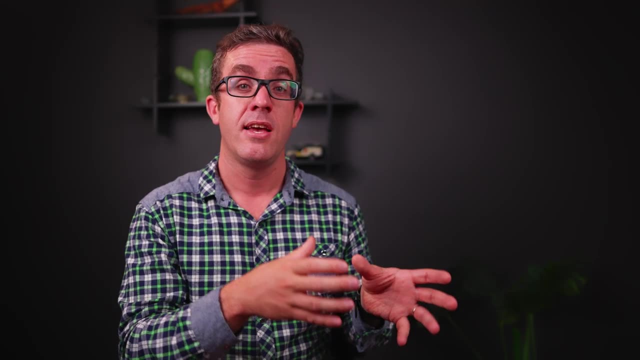 based on the soil type that you have. so if you've got a really good soil, such as the sand, you like to have minimal to no footings internally, where if you've got a really highly movable soil like a clay, you can add more footings into the system, stiffening it up. what are the different types of? 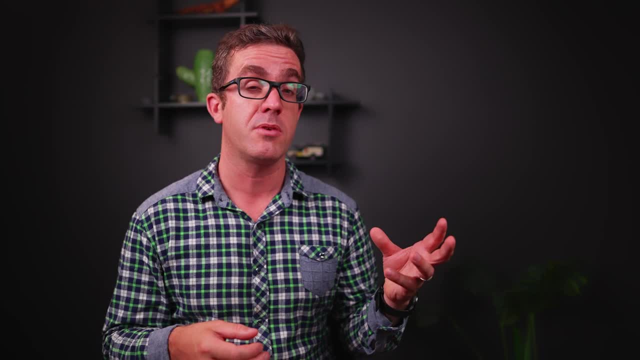 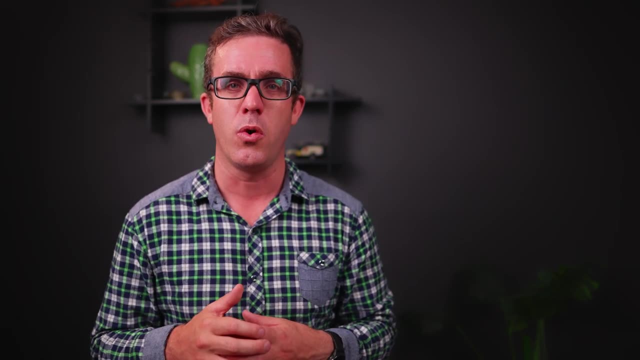 deep foundations they have available to you. so just say you've got really poor founding material, so you need to go down deeper, highly reactive soil that the building can't cope with. so you need to make sure the structure is stiffer or your loads are potentially just too high. the different types. 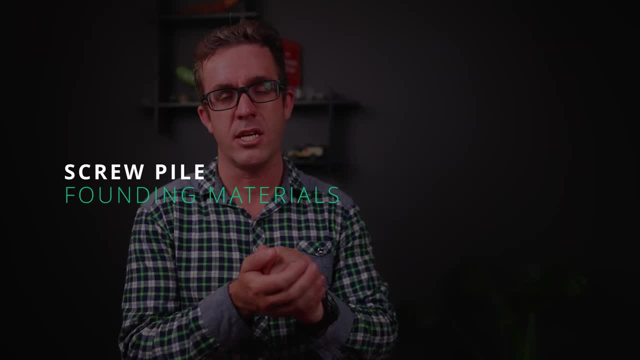 of deep foundations are available to you. so if you're going to have a really good soil type, then you need to start with the most easiest one first, which is your screw pile. a screw pile is essentially just a bit of steel with a propeller on the bottom that's screwed into the ground. so 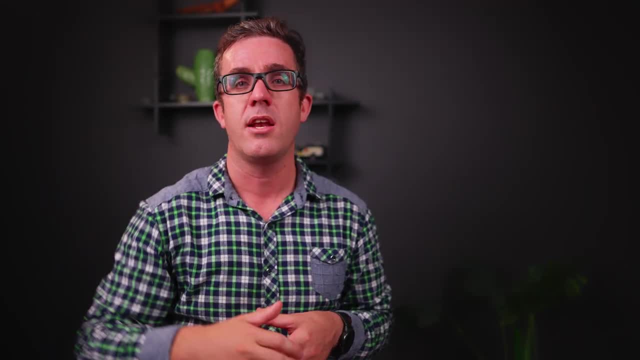 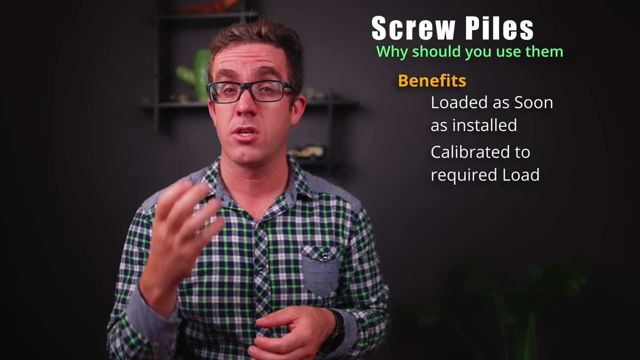 you can screw this down as deep as you can go, so it's quite easy and quick to install, as you essentially just get a machine, drill it into the ground and as soon as it's in place, it's ready to bear the material over. you can also calibrate it based on the load that you need, so sometimes you 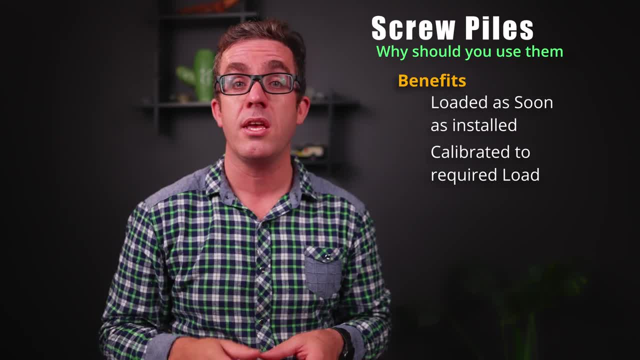 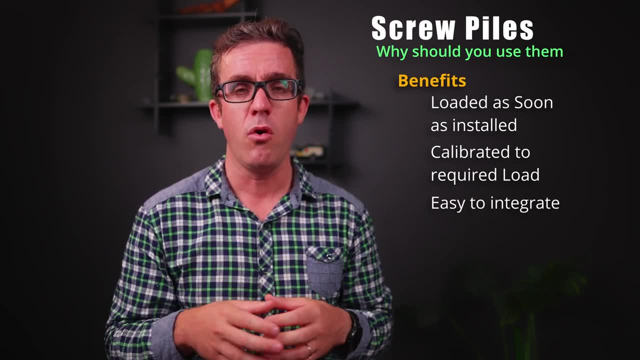 may need to go to a certain depth to get below the silt, but also based on the amount of torque that you need to apply to, it will be the given bearing capacity that you'll achieve out of each of those different types of footings. so if you're going to have a lot of work to do, you might want to. 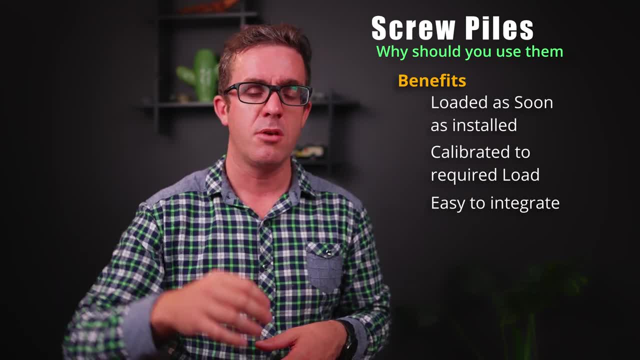 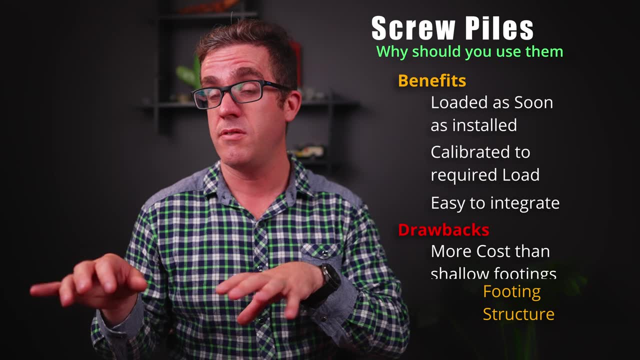 calibrate them. say, you've got a timber floor, you can just screw the screw pile into the ground and directly bear on top of it. but other times you may screw it a little bit further and either put a pad footing or strip footings underneath. now, of course, the footing system does get more expensive here. 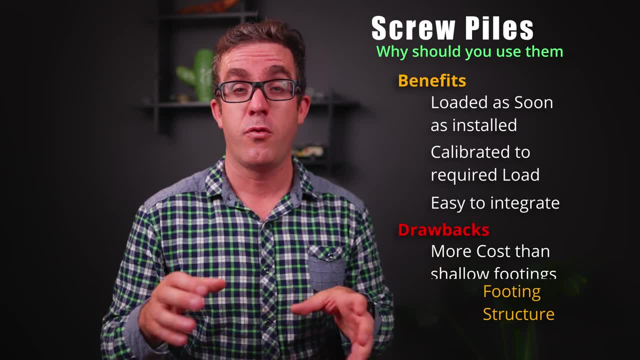 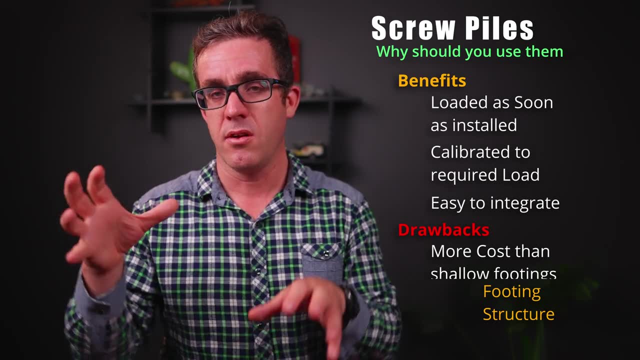 as, typically, the footing system needs a design to span between these different piling systems. it doesn't matter which one you choose. the footing system is suspended as it's bearing on these foundations that are a lot stiffer and a lot further apart. so not only do you need to pay for 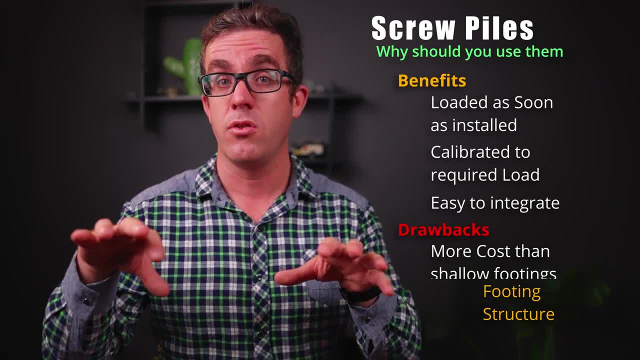 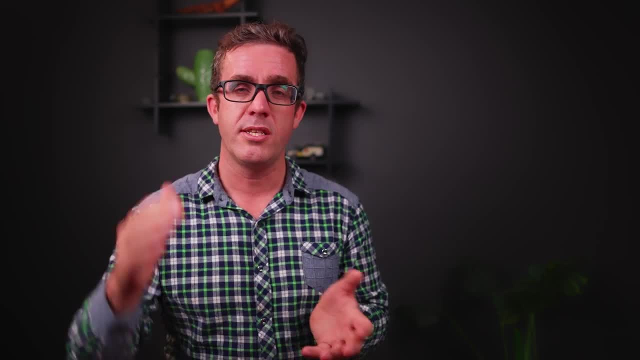 the screw poles or the piles, but you also need to pay for the increase in your stiffness of your structure over and allowing it to span between the supports. another type of foundation system that is very similar to that screw pole is that driven pile, so essentially you have a hardened pile. 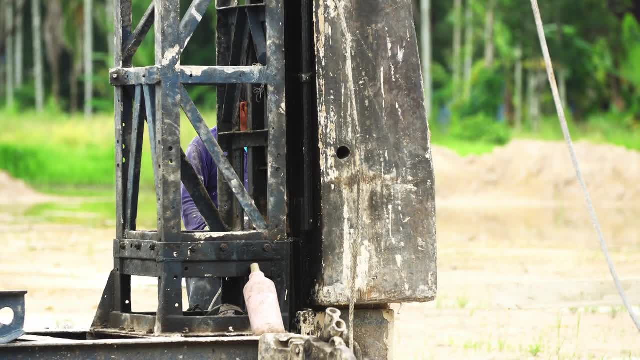 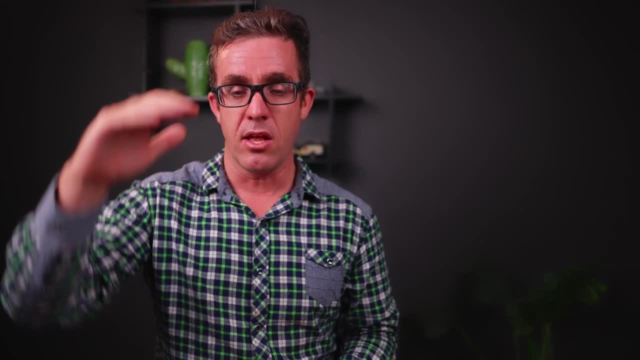 that's typically made up of a precast that will then be hammered into the ground. so as soon as you hammer it into the ground to the correct depth, it's ready to be loaded. now the problem with this type of system is this: impaction and concussion to get the footing system into. 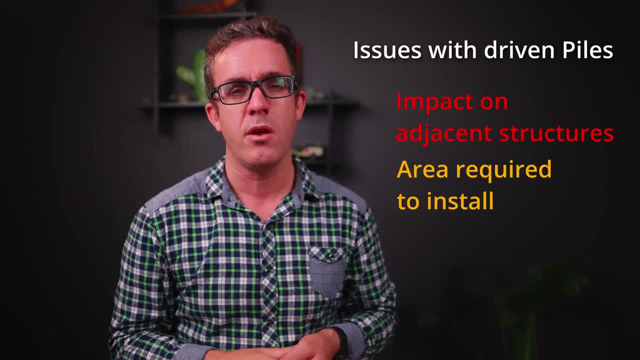 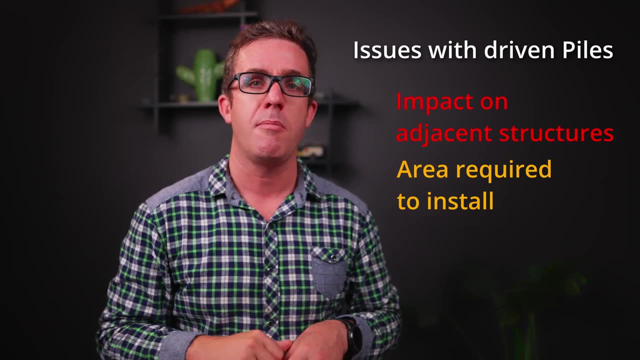 the ground potentially requires a bigger system with a lot of weight on top of it potentially shakes the buildings around it, as you can see big hammering motions banging into the ground that may vibrate the structure around it. that may cause problems for local residents, but typically it is better and quicker to build as it's already activated as soon as. 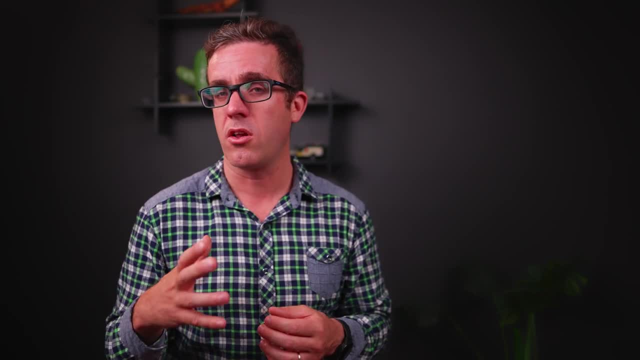 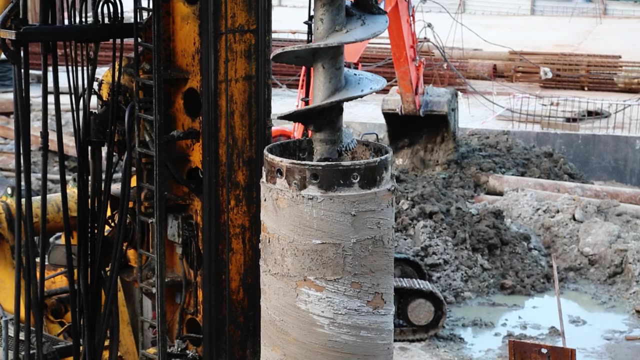 you've pushed it into the ground. the next type of foundation system you'll see quite a lot around australia and is that board pile or cfa piles. so essentially they get a big drilling rig out on site. so if you've ever seen those big constructions with those big drills, they're